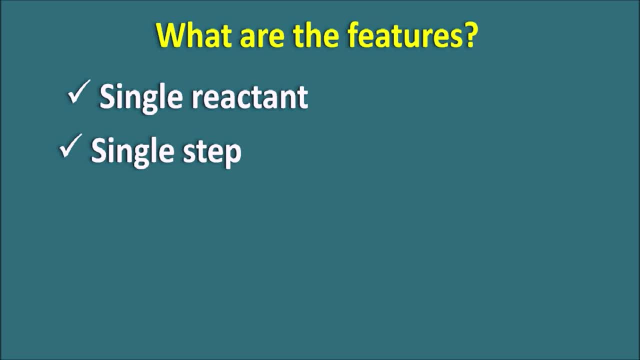 reactions, that means they will take in a single step. and third feature: the energy. these reactions requires energy and this energy can be supplied in the form of either thermal energy or photo energy. we can use the heat, otherwise we can use the UV radiation in order to produce the reaction and, interestingly, based on the 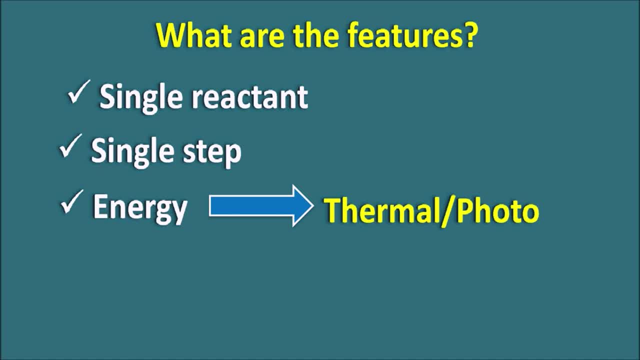 source of energy. whether we are using a thermal or photo energy, the configuration of the product will be fixed. so the configuration of the product depends on the source of the energy we are going to supply, whether a thermal or photo energy, as well as the number of pi bonds present in the 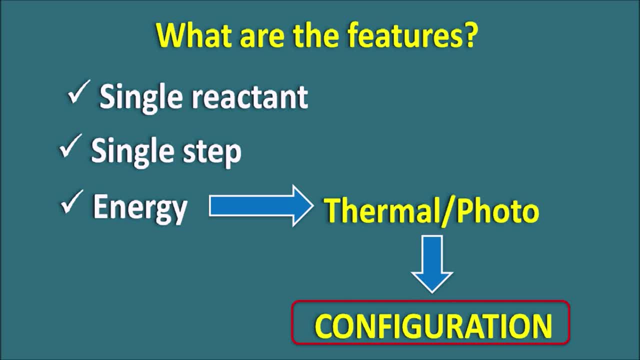 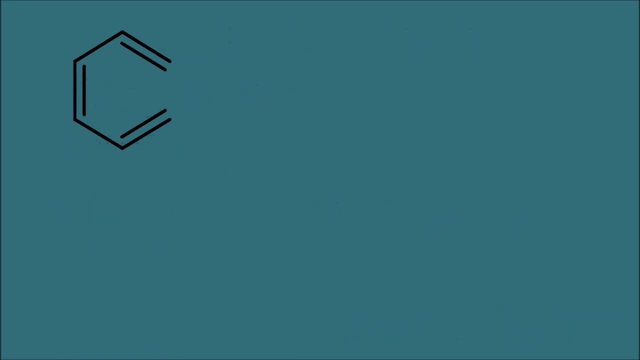 reactant. so today, in this video, let us see how this electrocyclic reaction takes place and different examples for this reaction and how the source of energy can affect the configuration of the product. so let us take with significance, simple example. here we have taken a compound. What is the nature of this compound? This 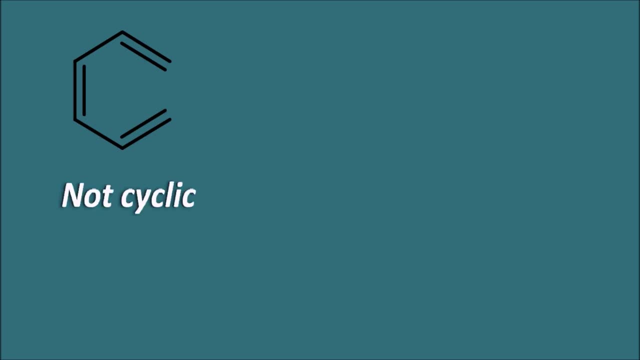 is not a cyclic compound because we can observe a opening there and it is having the three pi bonds, So it is a 1, 3, 5 hexa triene. It is an acyclic compound. In order to close the ring, we have to introduce a sigma bond here, and this cannot be achieved directly. 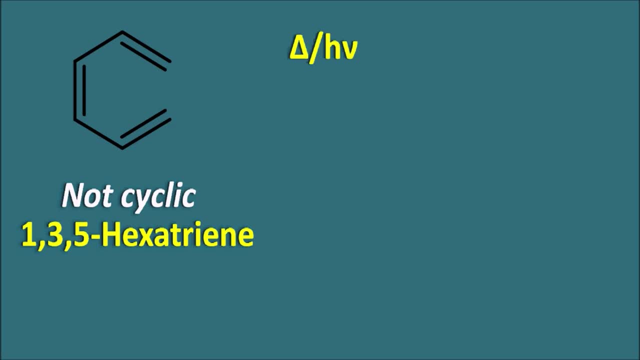 So when we supply the energy in the form of thermal or photo energy, the electrons can be delocalized, such that the electrons are delocalized, for example, here the pi bond can be converted to sigma bond and here this pi electrons can be delocalized to this position. 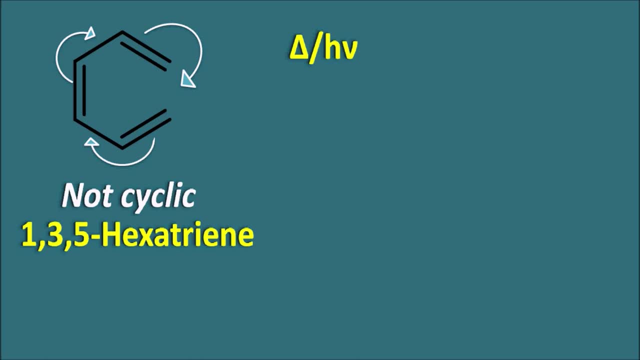 and here they can be shifted in this way. In this way, in a cyclic fashion, they are going to be rotated, where two pi bonds are going to be delocalized, but one pi bond is going to be converted into a new sigma bond. Now this 1, 3, 5 hexa triene on supply of energy. 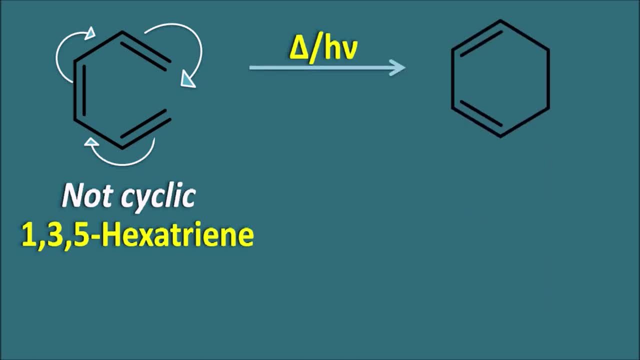 can be converted into one of the compound. What is the name of this compound? You can see that the two pi bonds are going to be delocalized there and it is nothing but the cyclohexadiene. And you can also observe that we have taken a triene, a compound with three double bonds, but now we are getting 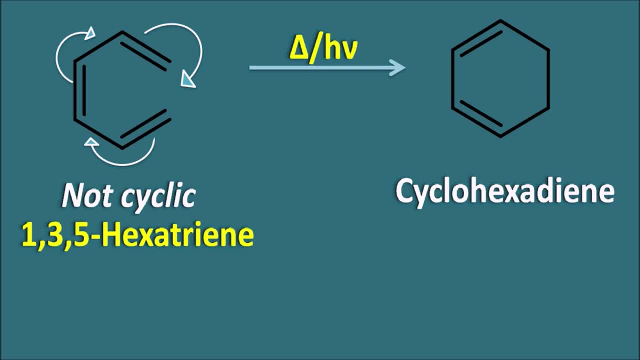 a product with only two double bonds. We are getting a diene, So one pi bond is going to be converted into one new sigma bond. So such type of reactions what we call electrocyclic reactions. But these electrocyclic reactions are also reversible in nature. So 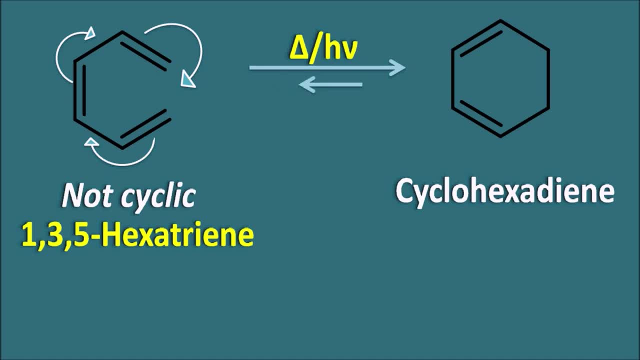 cyclohexadiene can also be converted into 1, 3, 5 hexa triene. But when we supply the sufficient energy, we can convert the reactant into the product. Now you can observe that here the hexa triene- three pi bonds are there- which is going to be converted into cyclohexadiene. 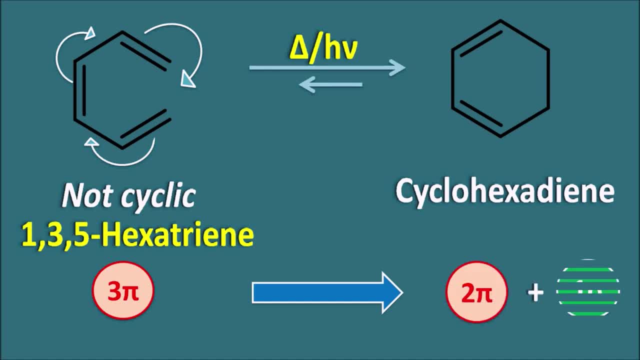 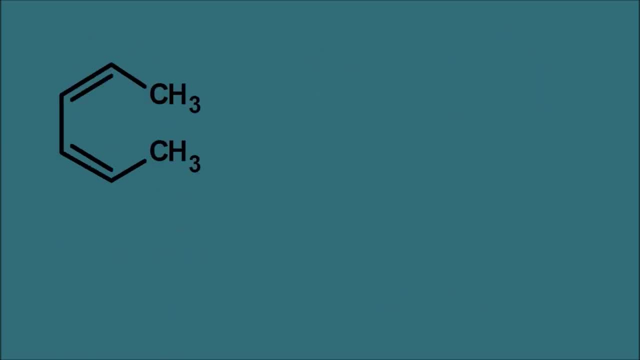 Now the cyclohexadiene is having two pi bonds, along with formation of a new sigma bond. Now let us take another example. So this is a diene having two double bonds, but these double bonds are not present at the terminal. So this is the 2- 5 hexa triene. So this is: 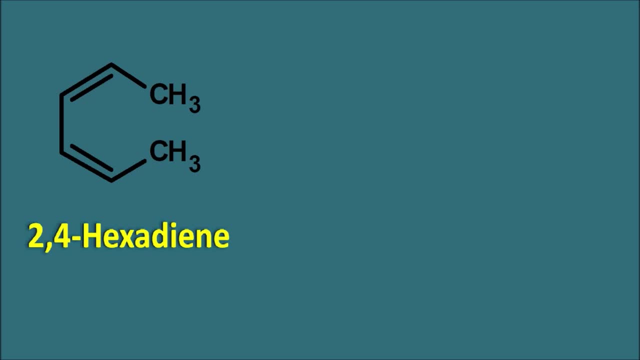 2, 4 hexadiene. Again it is having the six carbons, but the double bonds are present at the second and fourth position. Now how it can undergo the electrocyclic reaction. We should not confuse that here the sigma bond is going to be formed between these two carbons. 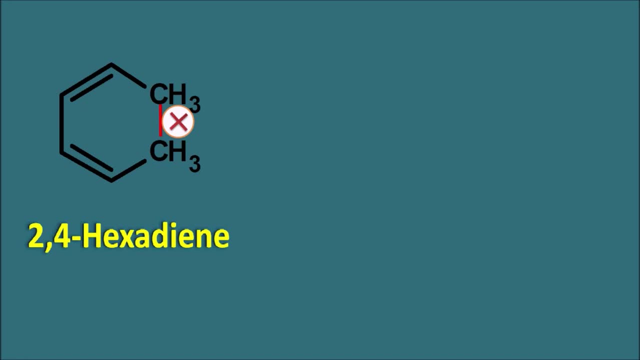 in order to close the ring. Since these carbons are not directly attached to the double bond, the new sigma bond will not be formed between these two carbons. So this is not correct. but we can see that one of the sigma bond here can be shifted to this carbon and here: 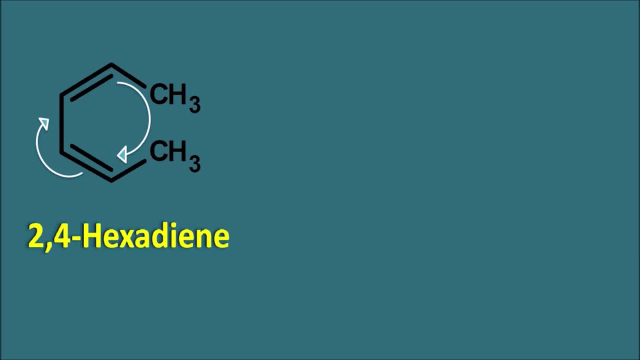 be shifted in this way so that they are undergoing a electro-cyclic reaction in presence of thermal or photo energy, to produce a product like this. Now you can see here the product is a cyclic structure with four carbons and other two methyl groups are outside the ring. So here the reaction. 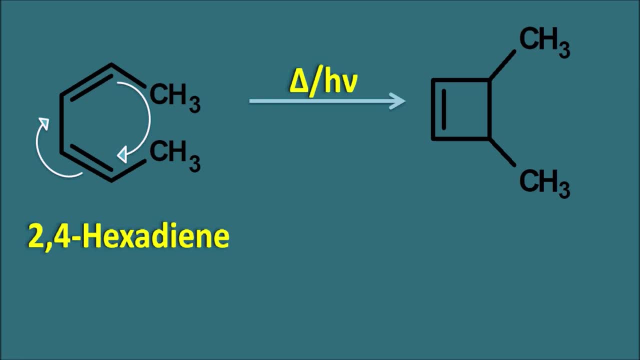 takes place between the four carbons which are having a conjugated diene system, and they are going to close the ring in order to produce a cyclobutene. So what is the name of this product? So the name of the product is nothing but the 3,4-dimethylcyclobutene. 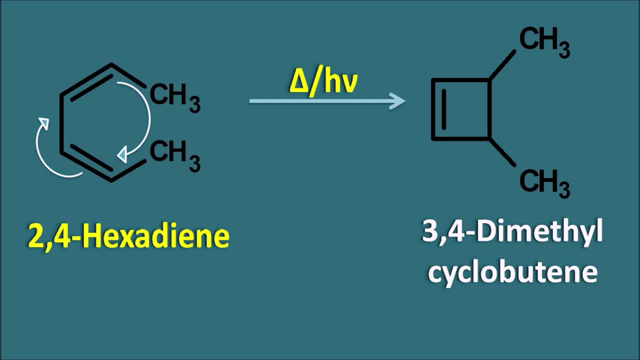 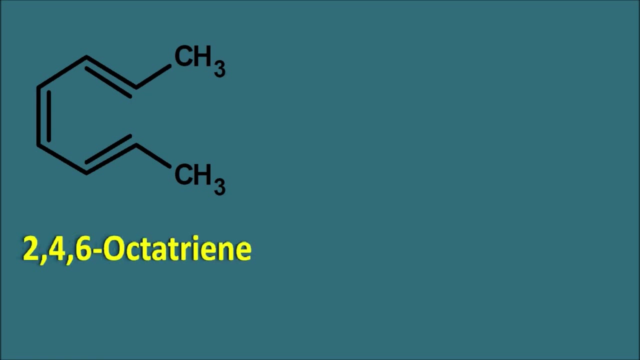 In this way, we have to carefully write the product in the electro-cyclic reaction, but again, this reaction is reversible in nature, so that this 3,4-dimethylcyclobutene can also be re-converted into 2,4-hexadiene. Now let us take another example. So this is the 2,4,6-octetrine. 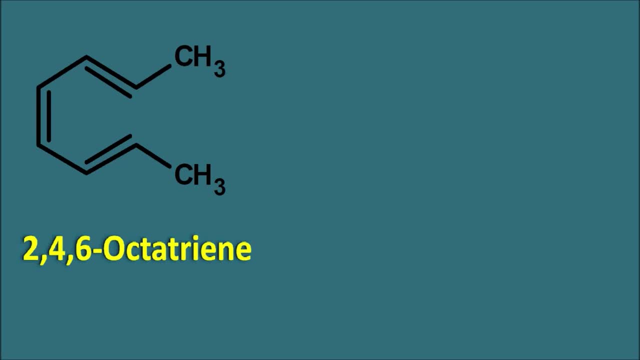 Now it is a 2,4-octetrine that is going to be converted into this 0,4-hexadiene. Now it is a having the three double bonds and let us see what happens to the configuration when it is reacted. 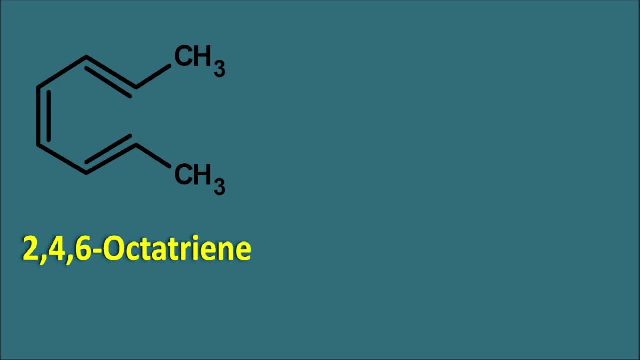 with the either thermal or photo energy. again, we should not confuse that the bond is going to be formed between these two carbons. this is not possible. but here, when we supply the thermal or photo energy, the reaction will take place at these positions such that this pi bond is coming. 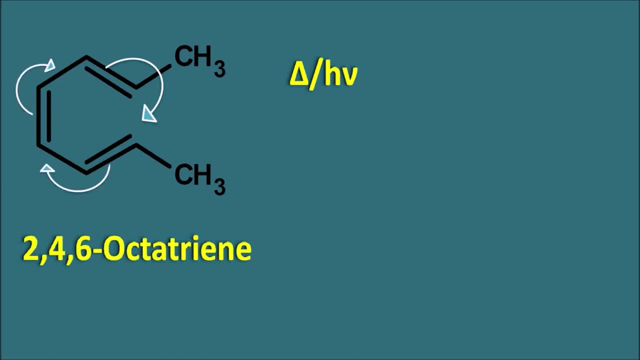 to sigma bond and this pi bond is going to be delocalized. and again, this pi bond is going to be delocalized to the ads and carbon, so that it is going to form a product which is a cyclohexadiene with the two methyl groups. now, this is nothing but the 5,6 dimethyl cyclohexadiene. now let us 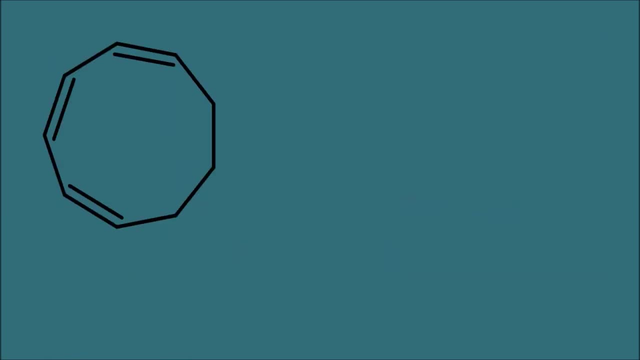 take another example, and this is a large structure, and when this structure is undergoing the electrocyclic reaction in presence of heat or photo energy, what will be the product? so let us see how we can write the product for this compound. first of all, let us give the 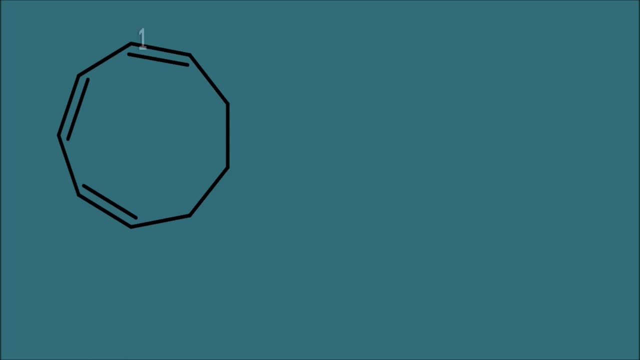 numbering to this cyclic structure. so we can start the numbering from double bond one, two, three, four, five, six, seven, eight, nine, so totally it is having the nine carbons and three double bonds. so it is a non-otriene with double bonds at the first, third and fifth position. therefore it is 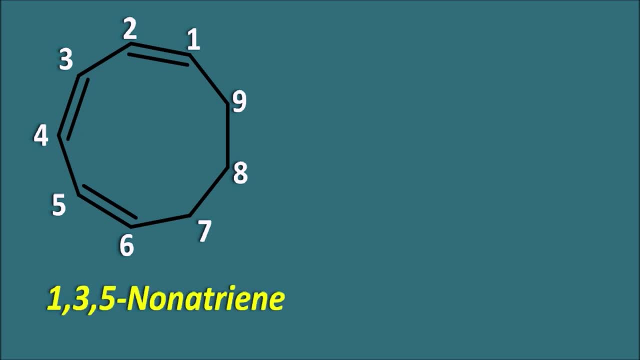 one, three, five non-otriene. now, this can undergo the electrocyclic reaction, just like we have seen the previous example. so when we supply the thermal or photo energy, it can undergo the electrocyclic reaction such that what are the pi bond between the cyclohexadiene and the electrocyclic reaction? 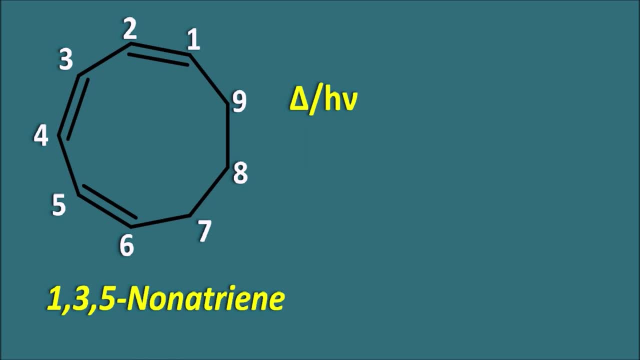 such that what are the pi bond between the cyclohexadiene and the electrocyclic reaction? the first and second carbon is going to be shifted to the sixth carbon, where this pi bond is going to be shifted to the ads and carbon, and finally, the ads and pi bond is. 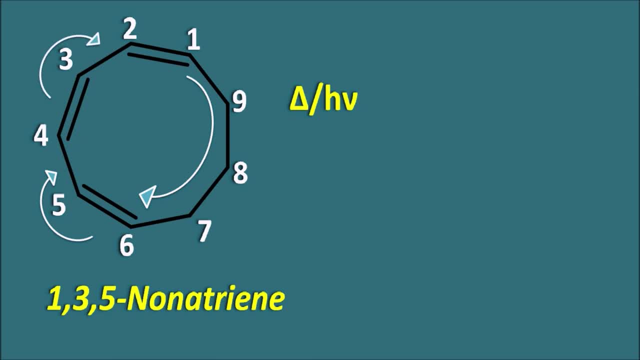 going to be shifted to the next carbon. in this way, again in cyclic fashion, they will undergo the delocalization where one pi bond is going to be going to new sigma bond and because of formation of new sigma bond, you can see that this monocyclic compound is now converted into a bicyclic compound. 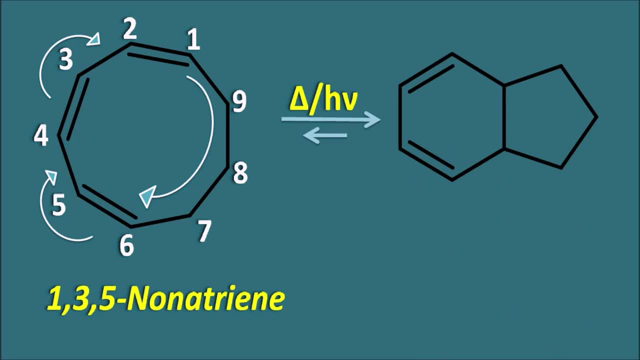 this will give a product like this. one of the cyclic is having the six member ring system with two double bonds, because here three pi bonds are initially involved in the reaction, and what are the other carbons which are not involved in the reaction are forming a five member ring system. 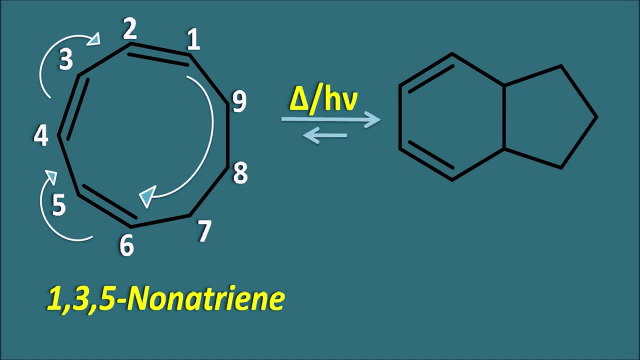 by fusion with this six member ring system- and here you can observe what are the ninth carbon, eighth carbon and seventh carbon are as it is and forming a five member ring system. in this way, by carefully observing the pi bonds, we can see that the six member ring system is now converted into a 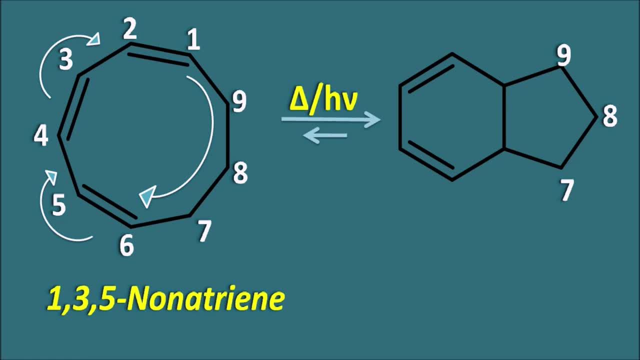 six member ring system. by fusion with these pi bonds we can easily write the electrocyclic reaction. so we have to just connect the terminals of the carbons which are having the pi bonds. but here these pi bonds should be conjugated. then only this electrocyclic reaction can takes place. 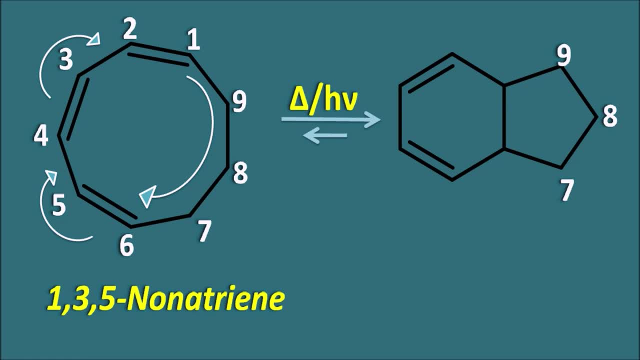 so that's about the electrocyclic reactions. electrocyclic reactions are the single step reactions and these reactions generally do not require any catalyst. and these reactions involve a single reactant which is undergoing a rearrangement in presence of a thermal or photo energy in order to produce a new compound with one new sigma bond and one less pi bond. 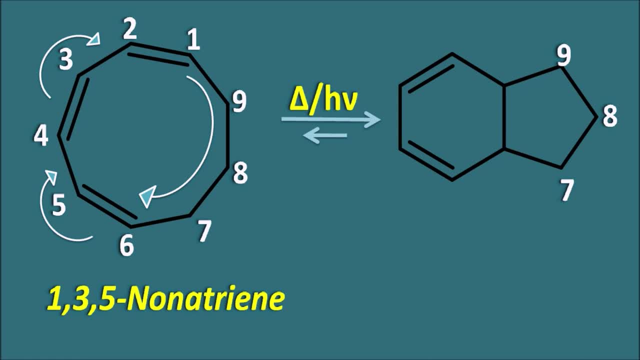 so here, a pi bond is going to be coming to a sigma bond in order to close the ring, and another important thing is that the reactant may be either a cyclic or cycling. in the first example, we have seen the cyclic dienes or trienes which are going to be coming to cyclic compounds by this. 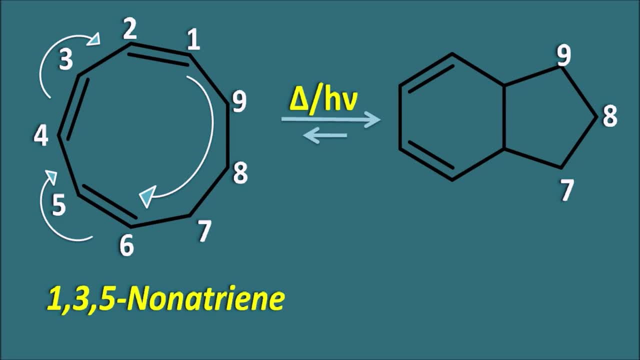 electrocyclic reactions. but in the last example we have seen, the reactant is initially a cyclic compound which can become a bicyclic compound on this electrocyclic reaction. so by this electrocyclic reaction, a new sigma bond is going to form which is going to close the ring. 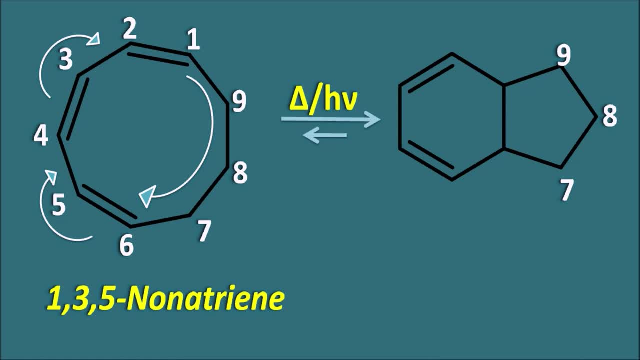 such that the number of rings are also increased. when we come to the configuration of the product, this configuration of the product depends on the configuration of the reactant, whether the reactant is having the double bonds, with either e configuration or z configuration, and how many pi. 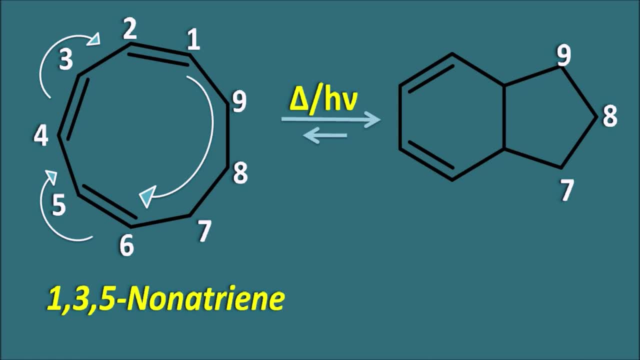 are there and by which source of energy they are going to be activated, whether the thermal energy or photo energy. by all of these factors we can fix the configuration of the product. in our next video we will see how can assess the configuration of the product by using simple tricks. so that's. 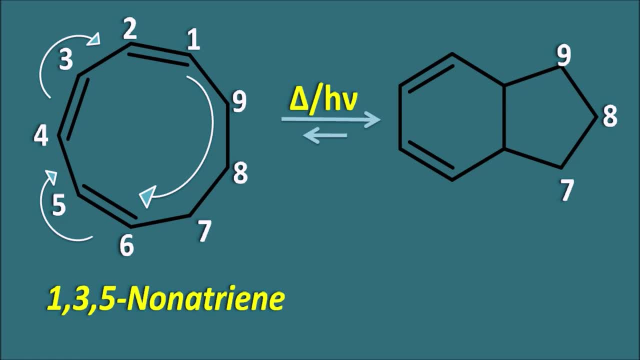 for today. if you like this video, please subscribe to our channel. share this video with your friends. post your comments in the comment box. thank you for watching this video.